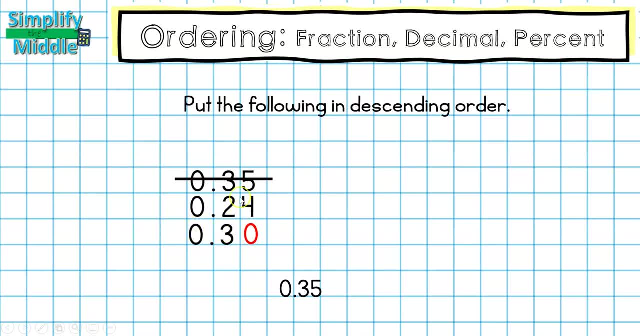 And then we know here that our three is larger than our two. so three tenths would be our next number, And then our last number, in descending order, would be our 24 hundredths. Now let's apply this to fractions, decimals and percents. 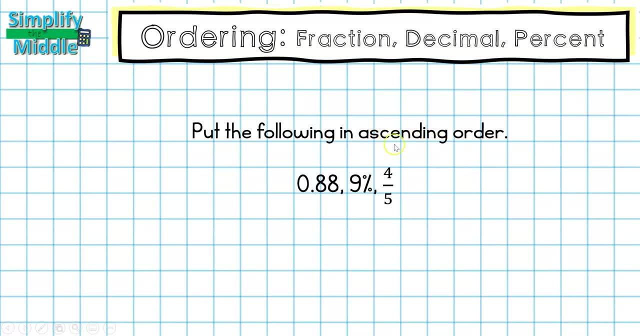 We want to put the following in ascending order, which means we're going to have three tenths, So we're going up, So we're going to look for our smallest number. Before we can do that, we need to convert all of these to the same form. 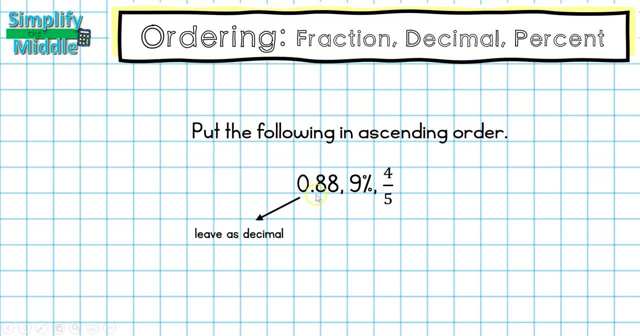 So I'm going to use decimal form. My 88 hundredths wouldn't change because it's already a decimal. I would change my 9 percent by converting and I would move my decimal place two places to the left. That gives me nine hundredths. 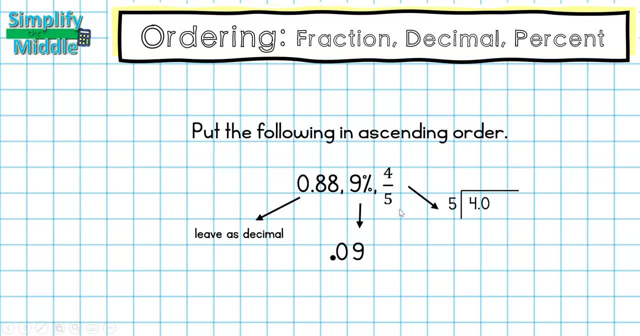 Finally, for my fraction, I would divide, I would divide using long division and I end up with eight tenths, Just like in the last example. I'm going to stack all of these decimals, But sometimes it's hard to remember which decimal goes with which number. 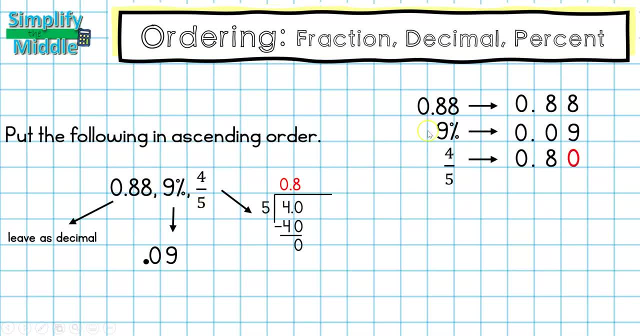 I always like to write them across from each other. That way I remember that eight tenths, for instance, is the same thing as four fifths. When I put them back into whatever order it asks for ascending or descending, I need to make sure that I use the appropriate order. 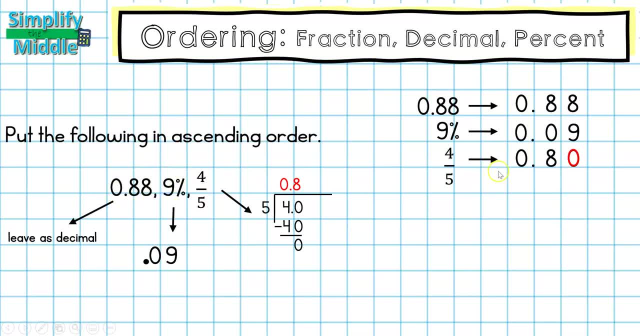 I need to make sure that I use the original numbers given in the problem, not the decimal conversions. Now, when I'm looking here, I see they all have zero for the ones place value. In the tenths place value I can see that this one has zero, while these two have eight. 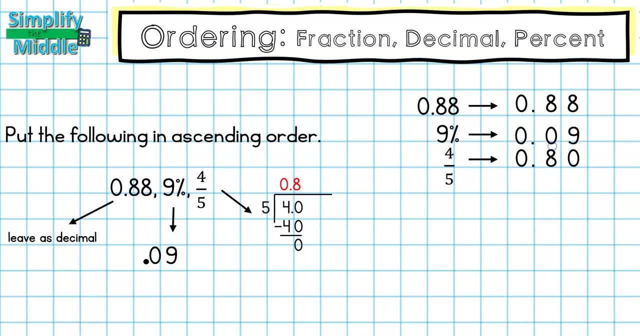 Since I'm looking for ascending order, I know that nine hundredths, or nine percent, is going to be my first listed number. Next I have 88 hundredths, with an eight in the hundreds place value, and eight tenths, which has eight tenths. 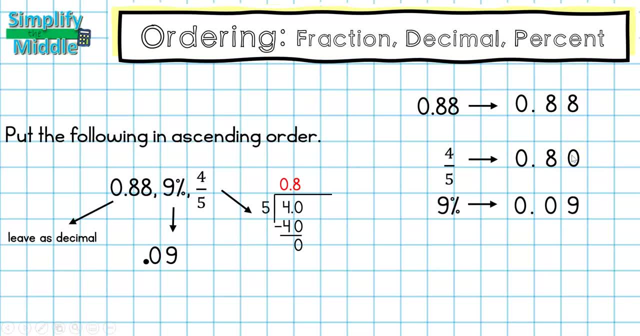 This one has a zero in the hundredths place value because it's the same thing as eighty hundredths. So I can see that four fifths, or my eighty hundredths, is going to be my next smallest number, And then that leaves my largest number as eighty eight hundredths.